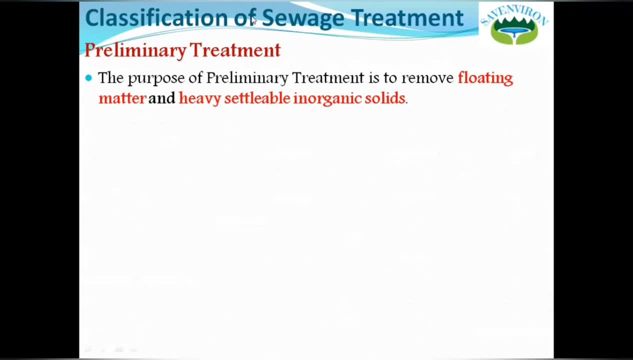 settlable inorganic solids. Preliminary treatment removes floating matters and heavy settlable suspended solids. Floating matter is like dead bodies of animals, pieces of wood, papers, rags, metal containers, plastic and rubber containers. All these things come. 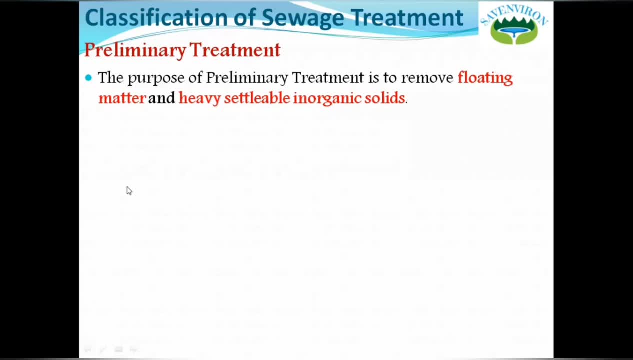 in floating matter And all these floating matter is removed in preliminary treatment, And these heavy settlable inorganic solids are sand, grits, bricks and pieces of wood are also removed in preliminary treatment. Then it also includes the flow measuring device, Preliminary treatment and flow measuring. 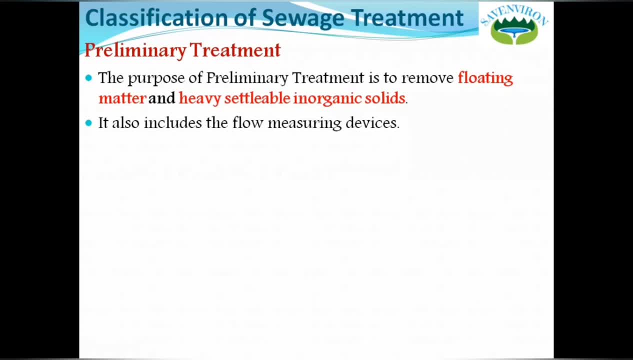 device are one unit, From which rate the flow rate increases, the flow rate decreases, and it also includes the flow measuring device, Preliminary treatment and flow measuring device. flow rate is also measured here if the floating matter and heavy settleable inorganic solids are not removed. 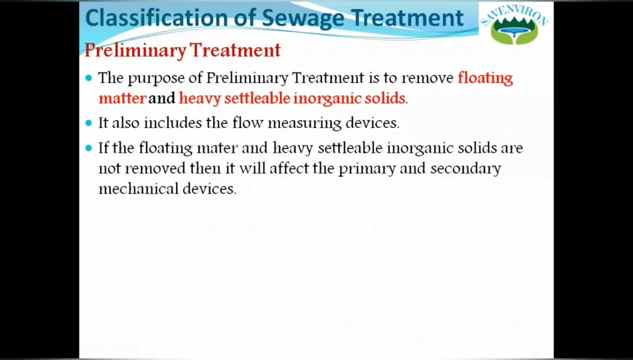 then it will affect the primary and secondary mechanical devices if the floating matter and heavy settleable inorganic solids are sanded. if this is removed, then the next treatment units- primary and secondary treatment units, such as mechanical devices like pump blades or aerators. chances of their deterioration will be very high. 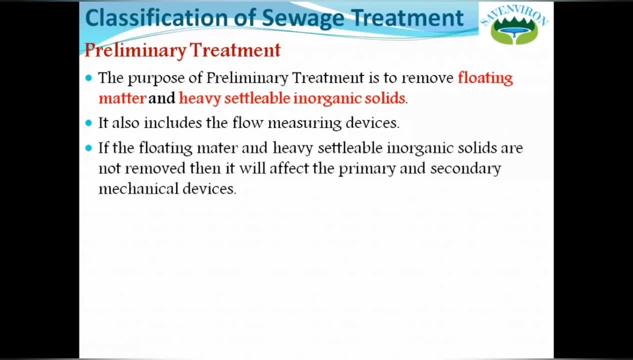 that is why we should remove all these things first, like settleable inorganic solids and floating matter. then it reduces BOD load of the waste water by about 5-10%. out of total waste water, 5-10% BOD load. only 5-10% of biodegradable organic matter is removed in preliminary treatment. 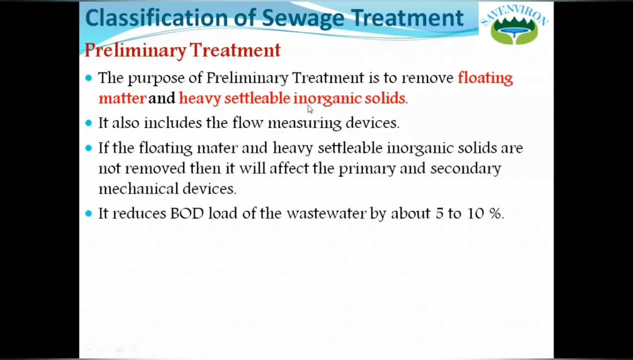 rest of the majorly inorganic solids are removed. units are removed. now what are the units in preliminary treatment? first is screens. in screen units, particles are removed, pollutants are removed, floating matter, maximum floating matter- is removed in screen. then grid chamber and detritus tank are removed in screen units. 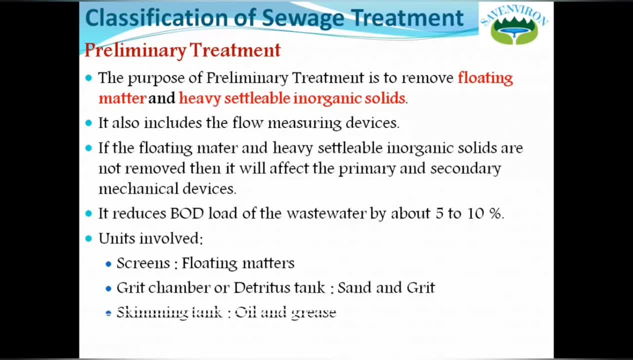 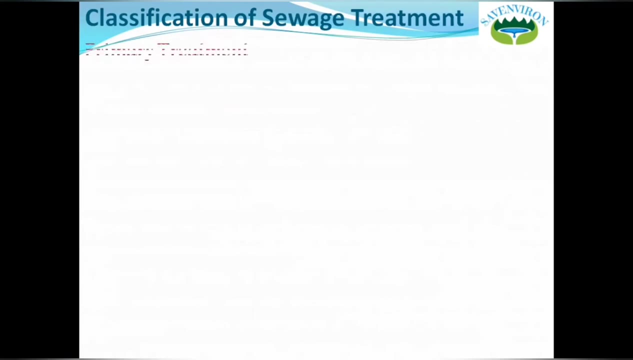 sand and grid are removed, then oil and grease are removed in skimming tank, then in combinators. in combinators the larger solids are grinded and chopped and converted into smaller size particles. then next is primary treatment. the purpose of primary treatment is to remove the large suspended solids. 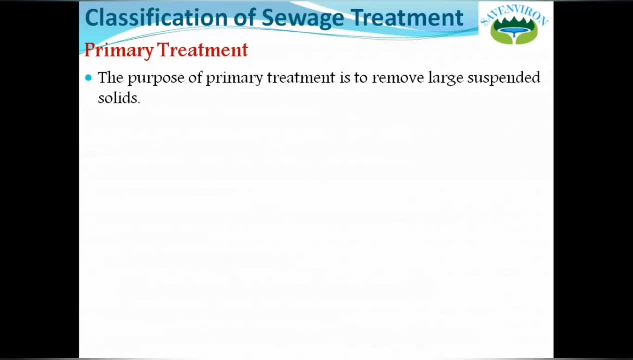 now what is there? first, floating matter is removed. inorganic solids are removed. now what happens in primary treatment? the large suspended solids are removed. if preliminary treatment is not given, then it removes organic as well as inorganic suspended solids. if preliminary treatment is not given, then the waste water will be directly in primary treatment. 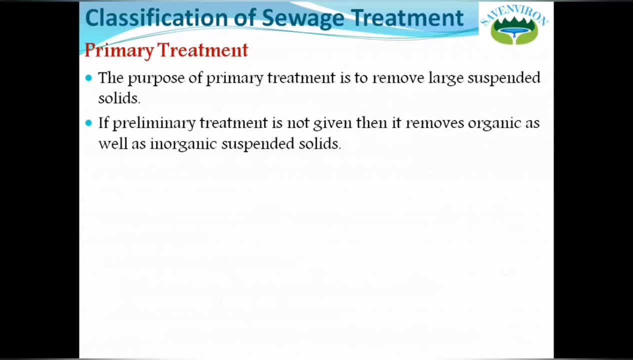 in waste water. inorganic solids are also going to be there. so where are the inorganic solids going to be removed? in primary treatment units itself. but when, when, when? when primary treatment is not provided, if preliminary treatment is not provided, if preliminary treatment is also provided. 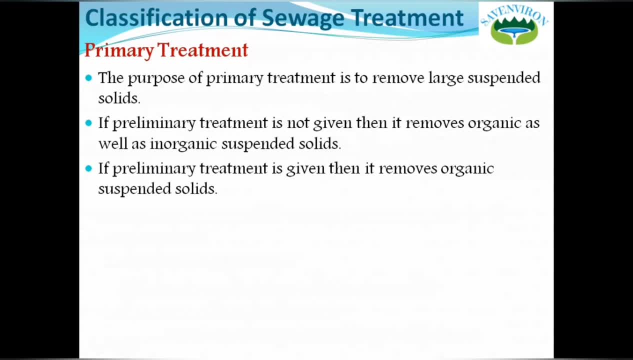 then what will happen is inorganic matters will be removed first in preliminary treatment. so what will primary treatment do? it will remove only organic suspended solids maximum. The units involved in primary treatment are sedimentation, large suspended solids, weight, specific gravity. Under the action of gravity, the large suspended solids will be settled and the primary treatment will be removed. 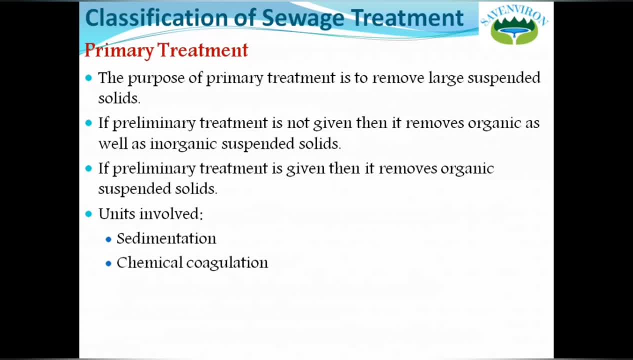 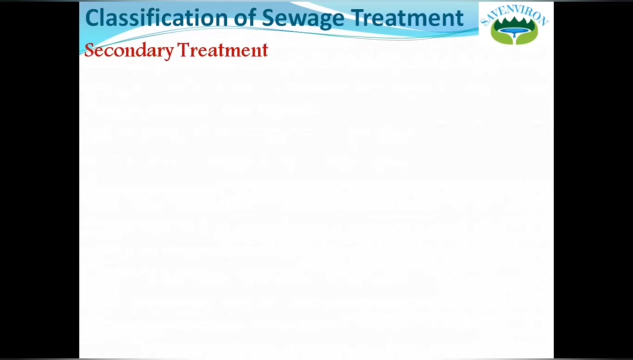 If we want to increase the rate of settling, we have to add chemicals. The chemicals added are called coagulant and the process is called chemical coagulation. Thank you. Next is the secondary treatment. Secondary treatment is the main treatment of any wastewater treatment plant or sewage treatment plant. 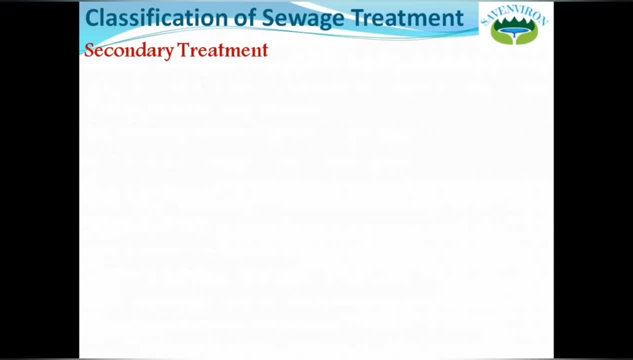 Secondary treatment is the main treatment part. It is also called as the heart of the sewage treatment plant or the wastewater treatment plant. The purpose of secondary treatment is to remove soluble and colloidal organic matter which remains after primary treatment. After primary treatment, the remaining soluble and colloidal organic matter is removed in secondary treatment. 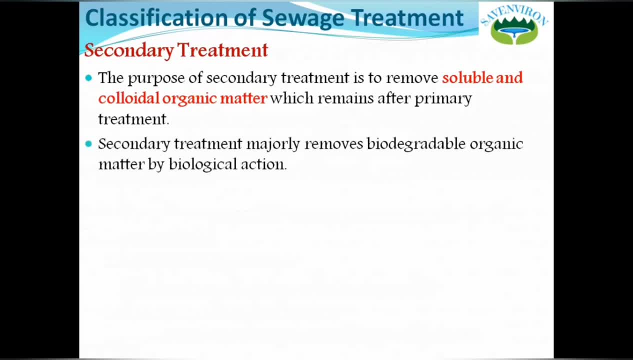 Secondary treatment majorly removes biodegradable organic matter by biology collection. What is removed in secondary treatment? Organic matter? Which organic matter The biodegradable organic matter is removed Through? which it is removed Through microorganisms and bacteria by biology collection. 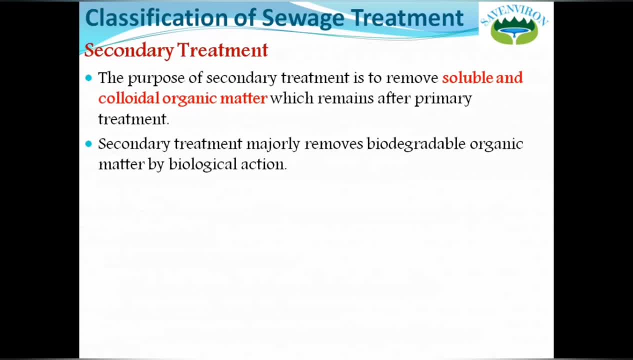 What will microorganisms and bacteria do? The biodegradable organic matter of the wastewater will be consumed. Biological treatment systems are designed to maintain a large active mass of bacteria within the system. Now what we have to do with biodegradable organic matter. 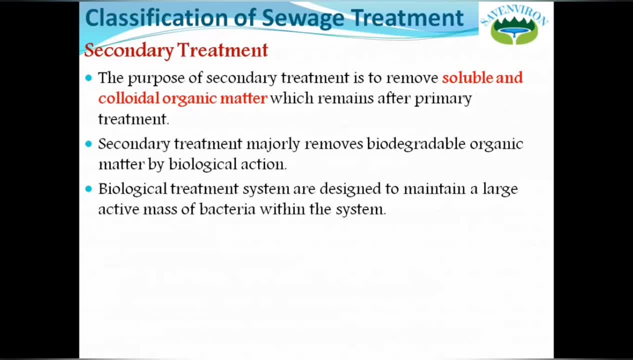 We have to trade it in secondary treatment According to which process it is going to happen, Which action is going to happen. It is going to happen through biological action, To have biological action in that treatment unit, in that biological treatment system. 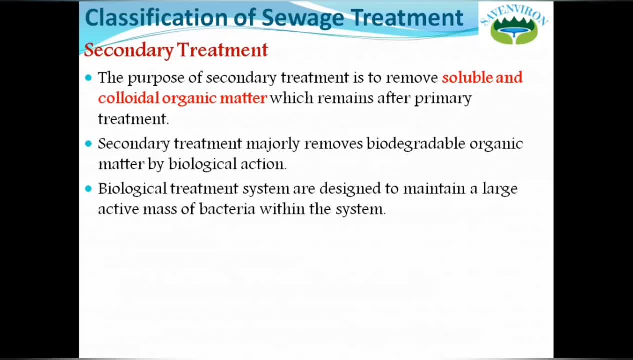 maximum number of bacteria, maximum number of microorganisms should be present. Only then the biological action will work effectively. Then secondary treatment process, classified as secondary treatment, is further classified as first is attached growth process. Attached growth process, as the name says. 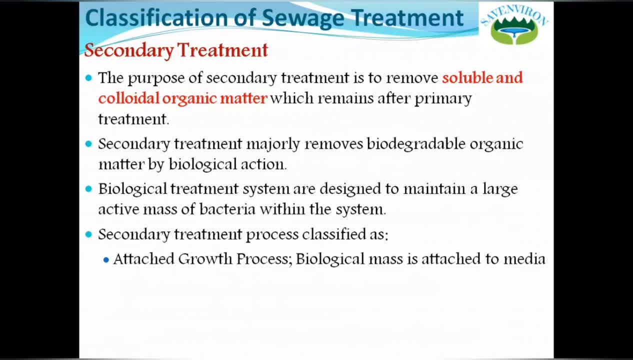 attached growth process In this the biological mass, bacteria and microorganisms. they will be attached to a particular medium. For example, take a sand filter. This is a sand filter. We will see this in the water treatment plant If in that sand filter. 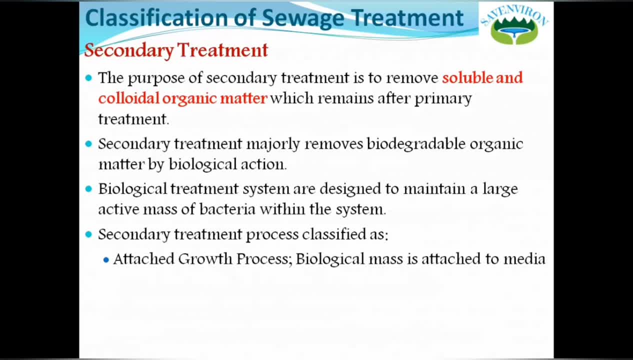 a biological mass, that is, microorganisms and bacteria. then what will they do for the bacteria? They will treat the waste water. So that type of treatment process is called attached growth process And that type of treatment unit is called. 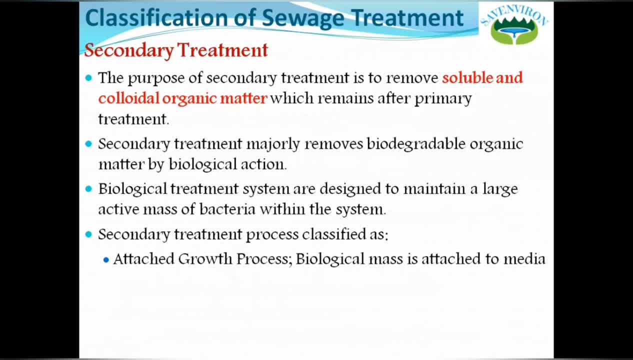 trickling filter. The example of attached growth process is trickling filter, Then suspended growth process. The name given in suspended growth process is biological mass. biological mass is going to be in suspension And the example of suspended growth process is: 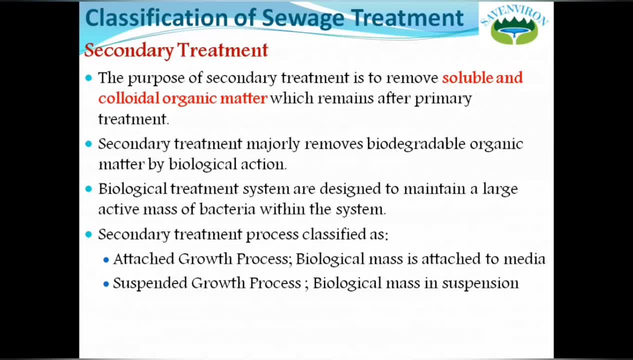 ASP activated sludge process, Then combined process. What will happen in the combined process? Attached growth process and suspended growth process will also come, And simultaneously both types of processes are going to happen: Attached growth and suspended growth will also happen. 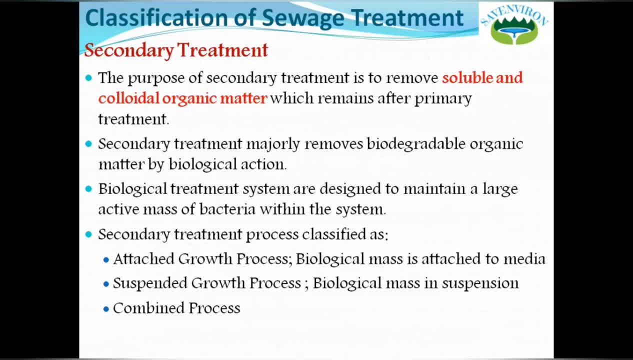 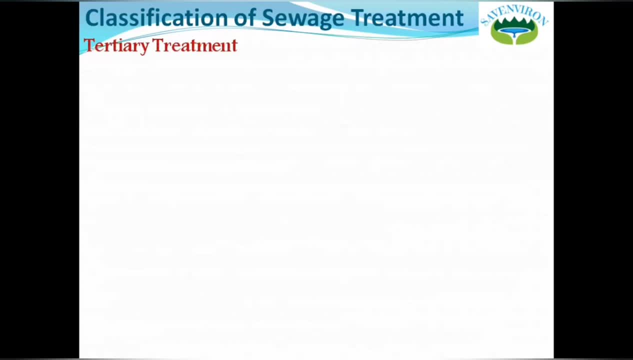 The example of this is amelial growth. Then tertiary treatment. Tertiary treatment is also called as the Advanced treatment. Now, what is the main purpose of tertiary treatment? First, I will tell you Now: Preliminary, Primary and Secondary Treatment. 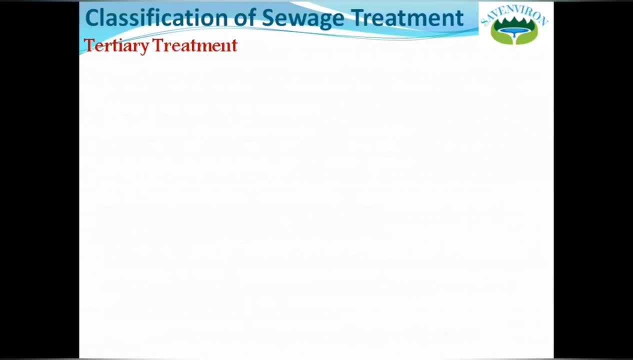 It is said that the maximum is removed. If we do not have treatment after this, then it will be fine, But we cannot use that sewage again Because there are many impurities in it Which will oppose the use of water. That is why we should not use. 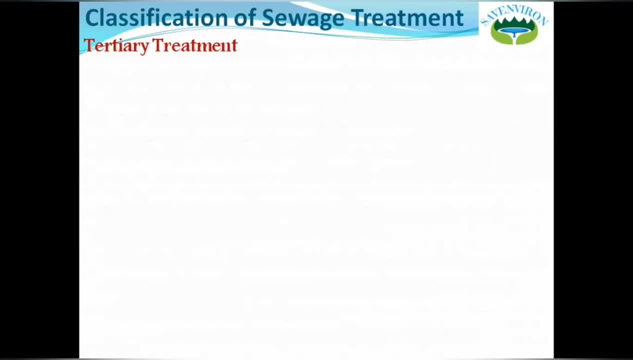 If we have to dispose only in the river or land, Then without tertiary treatment We can directly dispose the water After providing preliminary, primary and secondary treatment. But if you want to reuse the water Or enhance the quality of the treated sewage, Then we have to provide tertiary treatment. 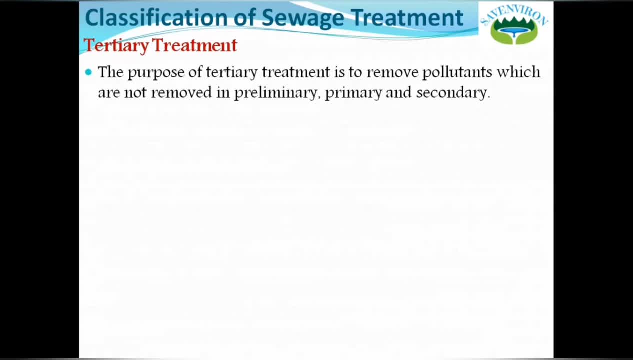 What is the purpose of tertiary treatment? The purpose of tertiary treatment is to remove Pollutants which are not removed in preliminary treatment, Primary, primary and secondary treatment, Which are not removed in primary, preliminary and secondary treatment, They will be removed in tertiary treatment. Tertiary treatment removes soluble inorganic compounds. 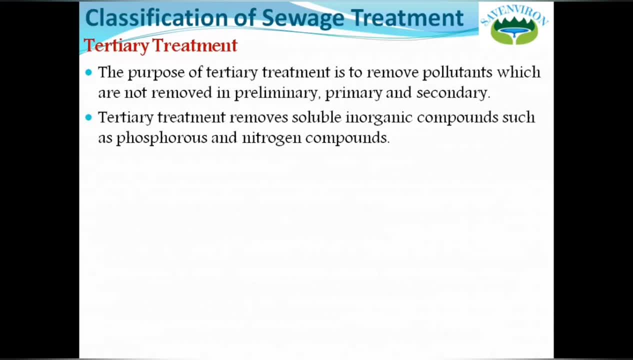 Such as phosphorus and nitrogen. Tertiary treatment removes soluble inorganic compounds Such as phosphorus and nitrogen And to remove nitrogen, The nitrogen which is removed from the wastewater Is removed from the biological exchange And there is no detention time. That is why tertiary treatment is provided. 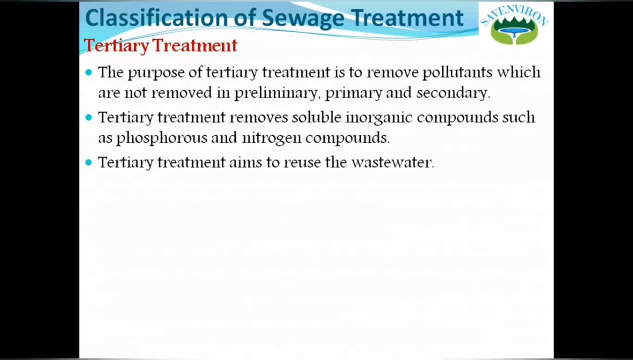 For phosphorus and nitrogen. Tertiary treatment aims to reuse the wastewater, But I have already told you, The main aim of tertiary treatment is To treat and reuse the wastewater. That is why tertiary treatment is provided. If we want to provide tertiary treatment, Then we simply provide disinfection. 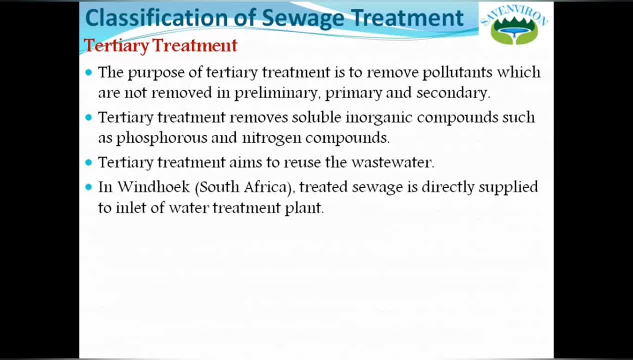 And then dispose the water. In Windhoek, A city in South Africa, Treated sewage is directly supplied To the inlet of the water treatment plant. What is said in South Africa? In a Windhoek city? The treated sewage, After providing tertiary treatment, That treated sewage- Is directly provided in the inlet of the water treatment plant. 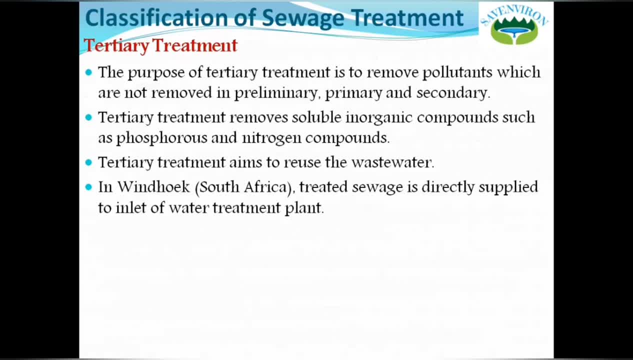 And there it is processed again, It is treated And it is brought to the drinking water quality standards And that water is supplied for drinking purposes. The main reason for this is In South Africa The water scarcity problem is very high. That is why In many places The treated sewage is directly 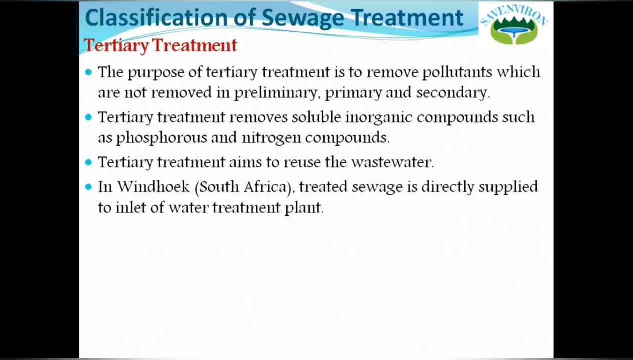 Provided to the inlet of the water treatment plant And once again it is treated well And then that water is utilized for drinking purposes. Then Tertiary treatment units involved. What are the treatment units That are seen in this? First is filtration, If we want to remove fine suspended solids. 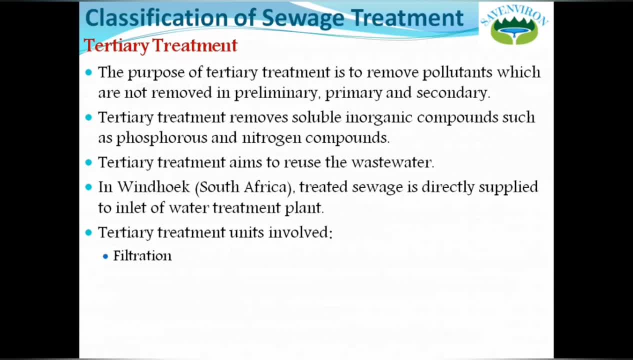 Then we have to provide filtration. Then Activated carbon adsorption. What is done in activated carbon adsorption? Soluble Organic And inorganic Particles will be removed, And then Odour and Colour can also be removed. Then De-mineralization: The minerals present in dissolved form. 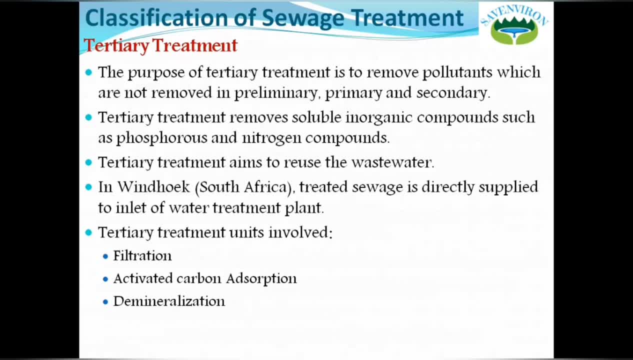 And the impurities present in dissolved form. What will happen in the de-mineralization process? Will be removed. Then Disinfection. What is in disinfection? In wastewater? The bacteria, Microbiomes, Virus, Harmful bacteria. What happens? What will happen to all of them? Will be removed in disinfection process.